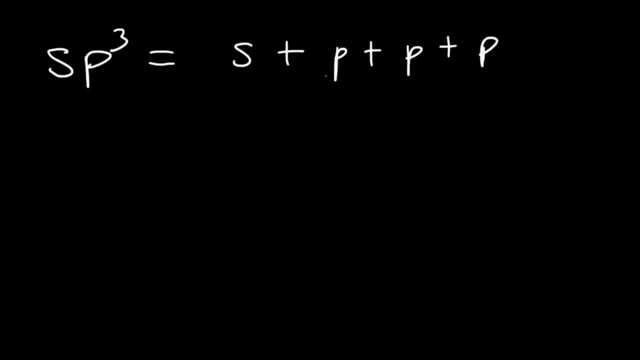 orbital and 3p orbitals. As you can see, it's s1p3.. sp2 squared is a hybrid of an s orbital and 2p orbitals. sp is a hybrid of s and 1p orbital. So now you. 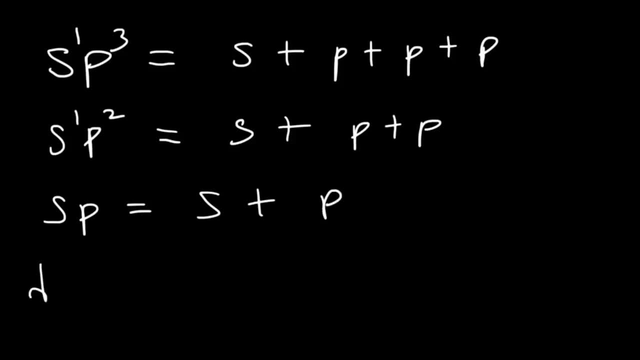 know what these terms mean. So let's say, if you were to see d2, sp3, this means that you're combining two d-orbitals, one s-orbital and three p-orbitals. So what exactly is an s-orbital, An s-orbital? 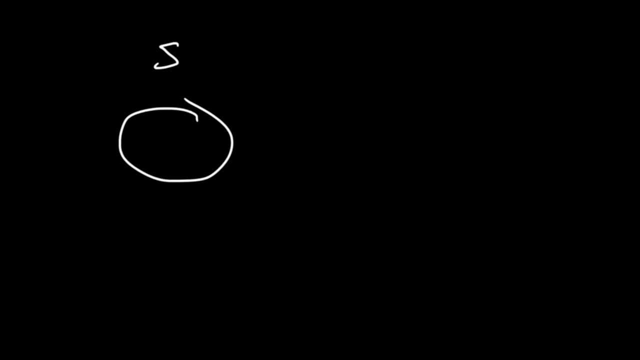 looks like a sphere, and an orbital tells you the probability of finding an electron somewhere within an atom. Keep in mind electrons. they can behave as particles and as waves. So an orbital simply tells you the most probable location in which you could find an electron. 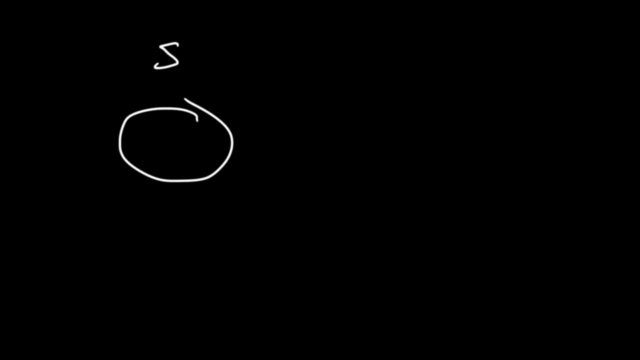 According to Heisenberg's uncertainty principle, we cannot know precisely the exact location of an electron. Now let's talk about the p-orbital. There's one s-orbital, but there's three different types of p-orbitals. You can have a p-orbital in the x-axis. 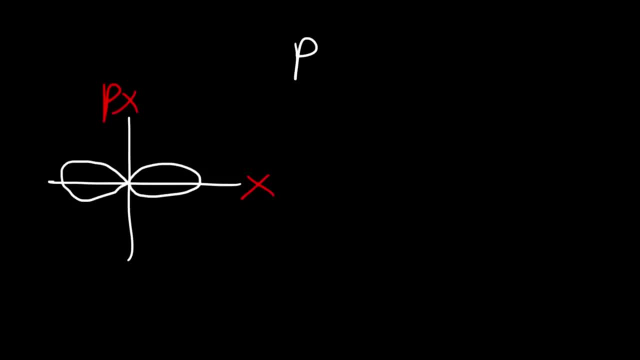 So this is known as px. You can have a p-orbital that's oriented along the y-axis, So that's called a py, And then there's one oriented about the z-axis, which we'll call pz. So there's three types of p-orbitals. Now we're going to talk about the hybridization of carbon. 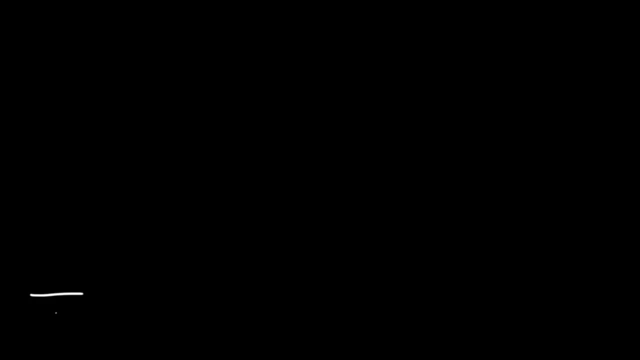 And the electron configuration of carbon is 1s2, 2s2, 2p2.. So this is the electron configuration of carbon. Now let's focus on this portion. Let's say the 2s is at an energy level here. 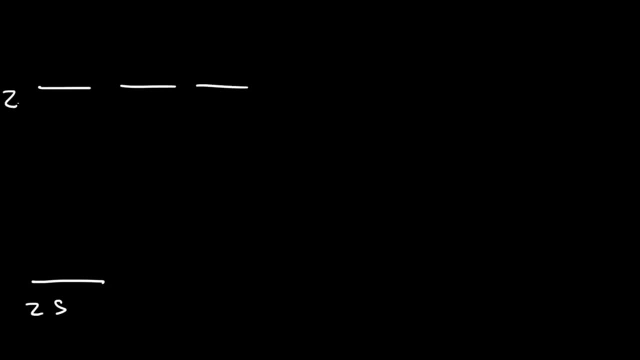 and let's say this is 2p. I want to highlight something. So carbon has four valence electrons. Now when carbon forms an sp3 hybrid orbital, it uses all four orbitals. Keep in mind: sp3 means that we need to mix 1s with 3p orbitals. 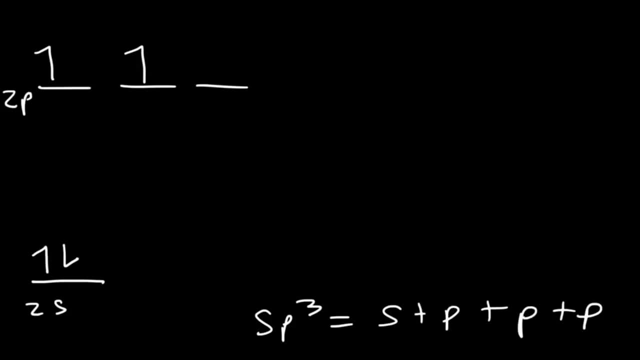 So where should we put the sp3 orbitals? Should we put them at the same energy level with the 2s orbital or with the 2p orbital, or somewhere in between, And should it be like halfway closer to 2s or closer to 2p? 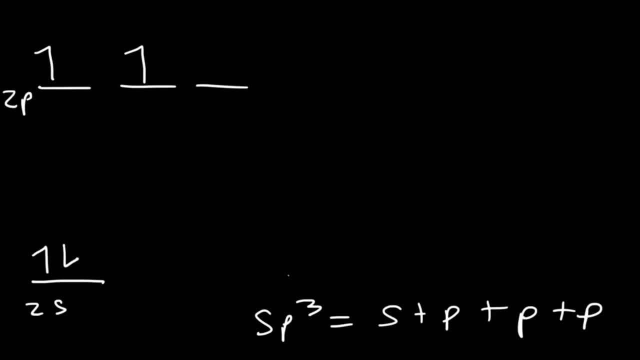 What would you say Now? to make an sp3 orbital, it requires four orbitals, as you can see here. So one out of those four orbitals is s, which means that the sp3 orbital has 4s. So that's the energy. 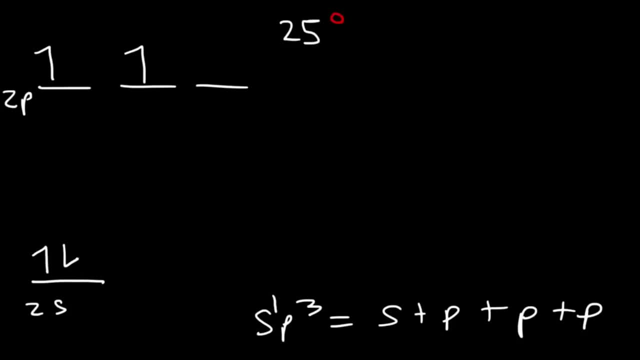 level you want to give to them. And if you want to make a 2s2 orbital, you need some energy and you need some s. So you just need an energy level. And now, if you put them 25% s character, Now there's three p orbitals out of four orbitals, Three out of four. 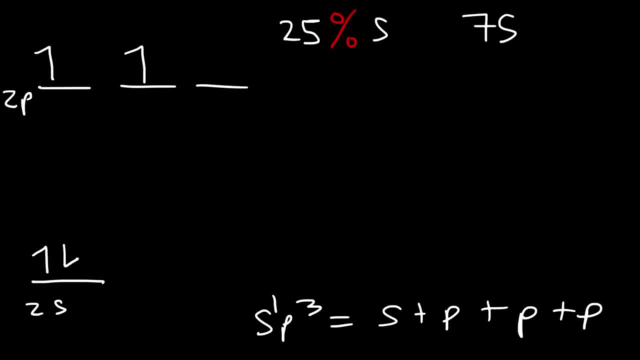 correlates to 75%, So there's 75% p character. So because the sp3 hybrid orbital has more p character than s, the energy level should be closer to 2p than it is to 2s, So it should be somewhere over here. Now, all four of these sp3 hybrid orbitals, they're called. degenerate orbitals. Degenerate orbitals are those that have the same energy. So these four electrons will be placed in these four sp3 hybrid orbitals And you want to place the electrons one at a time, when you're adding electrons to degenerate orbitals or orbitals of the same energy. 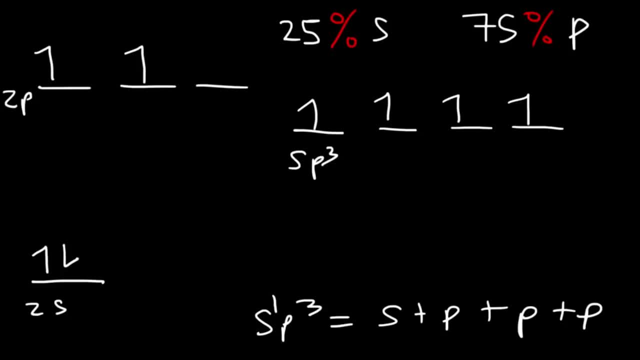 And that's the main idea behind Hund's Rule. You want to add electrons with parallel spins, one at a time, if you're adding them to orbitals of the same energy. Now let's talk about the sp2 hybrid orbital. Let's talk about its energy first. 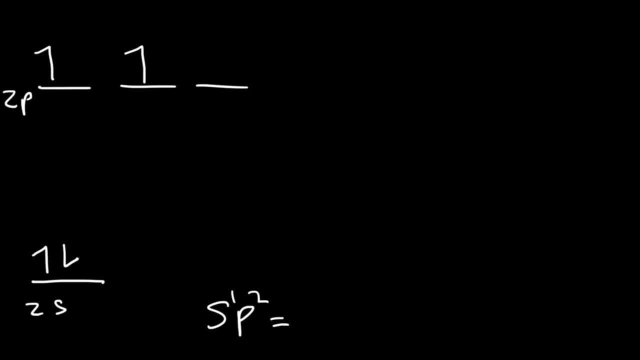 So to make an sp2 hybrid orbital we need one s orbital and two p orbitals. So we have three p orbitals. We're not going to use all three of them, We only need to use two. That means one of them will remain after hybridization. 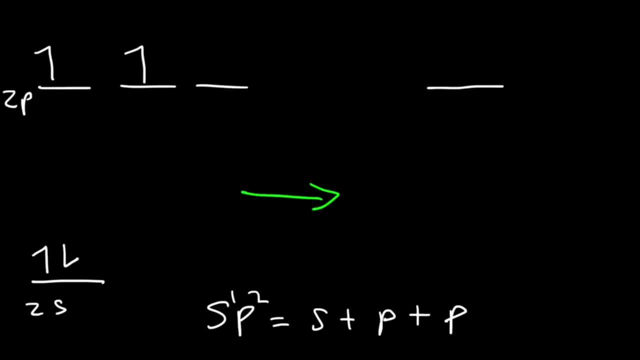 So the green arrow would represent the process of hybridization. So here's the unhybridized 2p orbital. It has the same energy, And now we have sp2.. So one out of the three orbitals is s, So we have 33% s character. 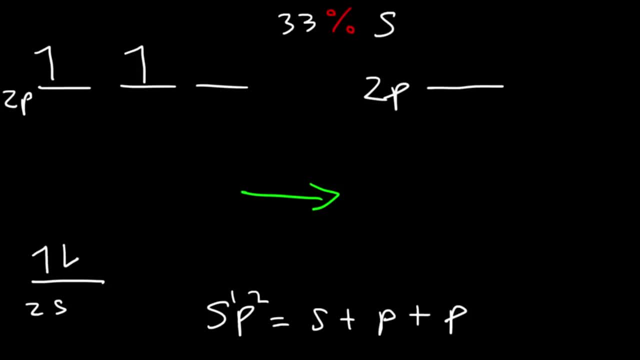 And two out of the three orbitals is p. Two out of three is about 67%. if you round it, So it's 67% p character. So we still have more p character than s. So therefore the sp2 hybrid orbital should still be closer. 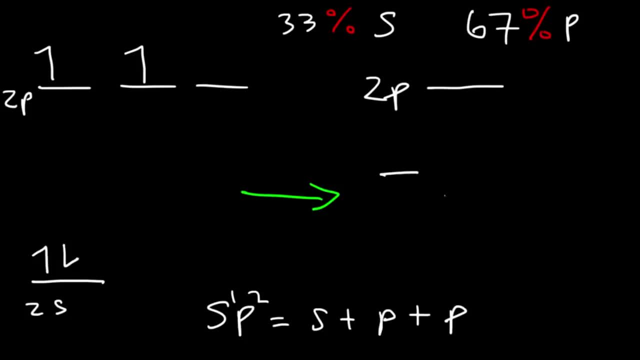 to 2p than 2s, But it should be less than sp3.. So these three orbitals will have the same energy. Since we used three orbitals to make them, we're going to get three hybrid orbitals, So I'm going to put one electron in each orbital. 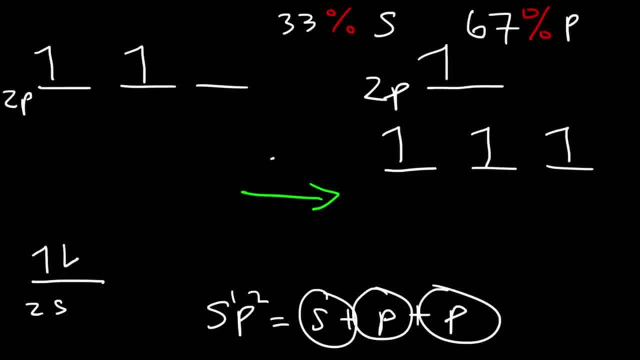 So we should have something that looks like this. So these are the three sp2 hybrid orbitals. Now let's talk about the sp hybrid orbital. So after hybridization, to make the sp hybrid orbital we need one s orbital and one p orbital. 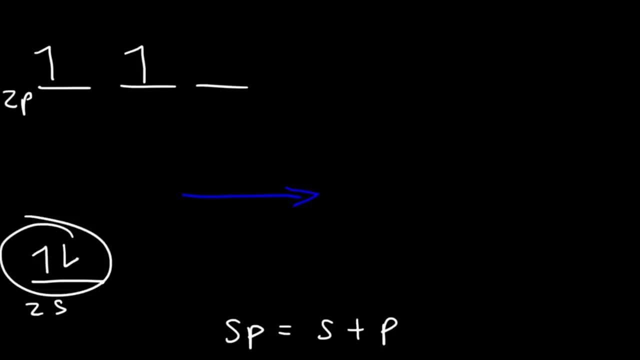 So we're going to use this s orbital and only one of the p orbitals, which means the other two p orbitals are unhybridized, So therefore they will be unaffected. Okay, Now, if we have an sp orbital, one is s and one is p. one out of two is 50%. 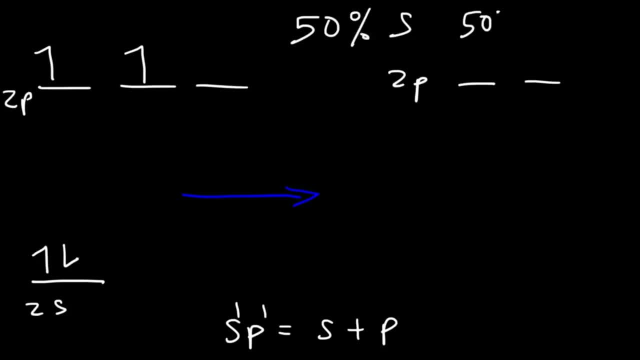 So therefore we have 50% s character and 50% p character. So therefore the sp hybrid orbital should be right in between the s orbital and the p orbital, And there's two of them, Since we use one s and one p orbital, or two orbitals to make the sp hybrid orbital. therefore, 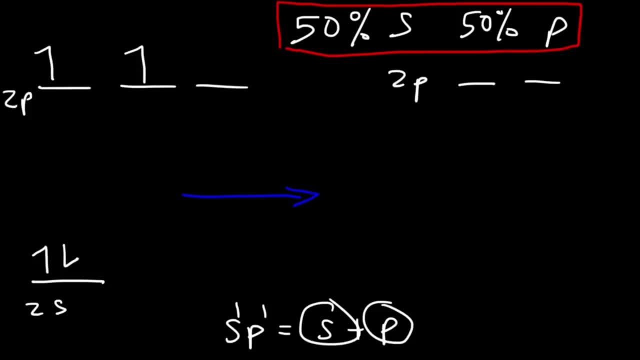 there must be two hybrid orbitals. So if you were to mix three atomic orbitals, you should get three hybrid orbitals. If you mix four atomic orbitals, you should get four hybrid orbitals. We're mixing one s and one p. 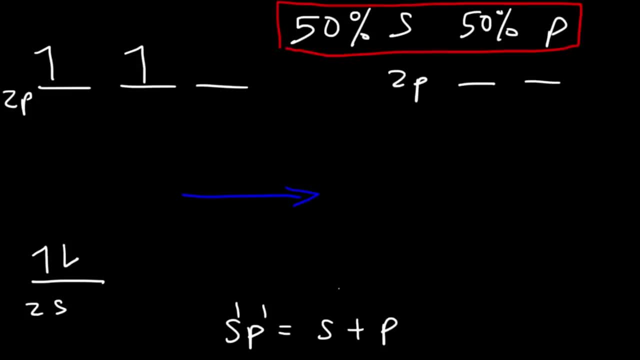 That's a total of two atomic orbitals. So that will give us two hybrid orbitals And they will have the same energy. By the way, you need to know that hybrid orbitals are used to form sigma bonds. Okay, Okay. 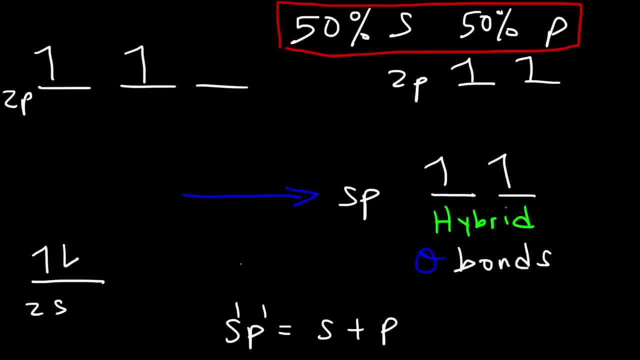 So the unhybridized orbitals, in this case the p orbitals that were unaffected- unhybridized orbitals are used to make pi bonds, which we'll talk more about later. So just keep that in mind. So pi bonds are always made from unhybridized p orbitals. when you're dealing with carbon. 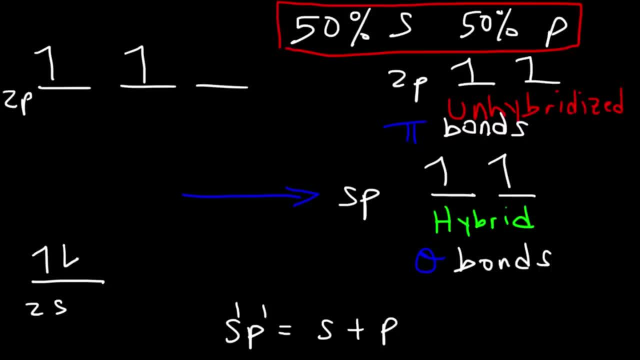 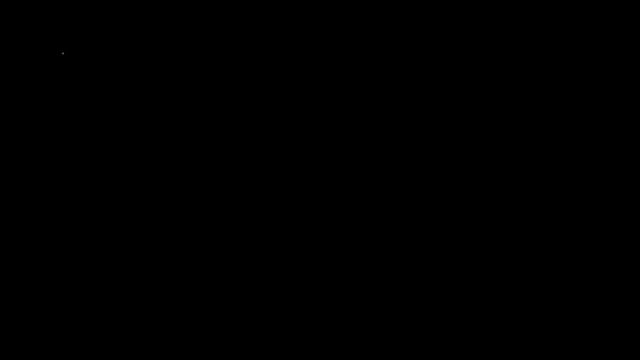 atoms And sigma bonds. they form from the overlap of atomic orbitals And they consist of pi bonds. Okay, So you can see that they are either one or two hybrid orbitals. for the most part, Every single bond that you see contains one sigma bond. 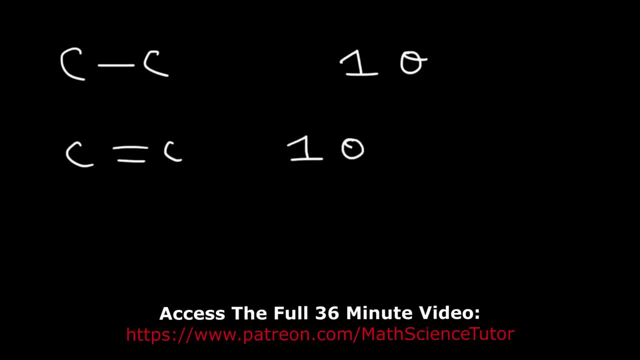 Every double bond has at least one sigma and it has one pi bond. A triple bond contains one sigma and two pi bonds. By the way, a triple bond is stronger than a sigma bond or a single bond. Okay, Three bonds are more stronger than one bond. 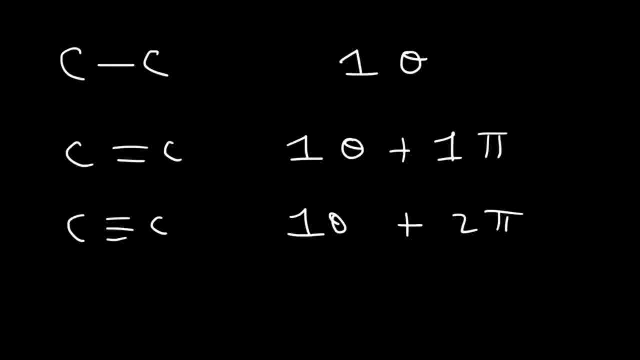 It's harder to break three pencils than it is to break one, So keep this in mind. triple bonds are stronger than single bonds, But triple bonds are shorter than single bonds. Single bonds are longer, But now, if you compare one bond to another, You need to know that. 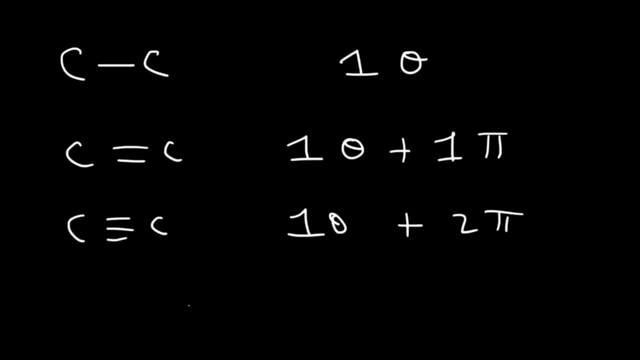 Well, before I say it, which one do you think is stronger, A sigma bond or a pi bond? What do you think about that? Sigma bonds are stronger than pi bonds. The reason why a triple bond is stronger than a single bond Is because you're comparing three bonds as opposed to one. 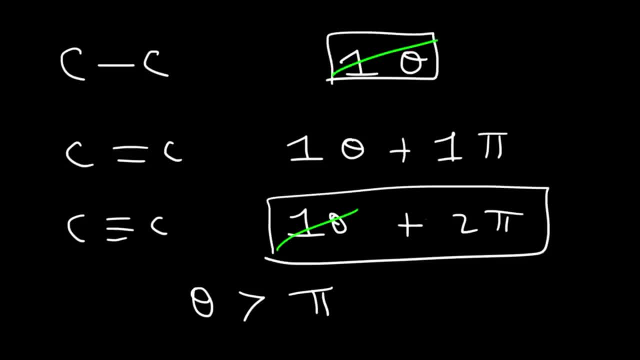 So these two sigma bonds- let's assume they're equal- The triple bond is going to win because it has two additional pi bonds. So when comparing a triple bond versus a sigma bond, The triple bond is stronger because you're comparing three bonds compared to one. But if we compare one sigma,